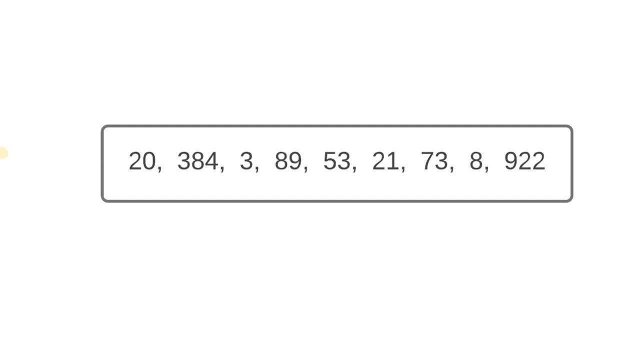 numbers to be sorted. Now, basically, this video is going to be divided into three sections. Alright. in the first section, which is the one we're on right now, I'm going to show you a work example of how Radix Sort actually sorts and an array- Alright. in the next part, we'll actually take a look at the code for the. 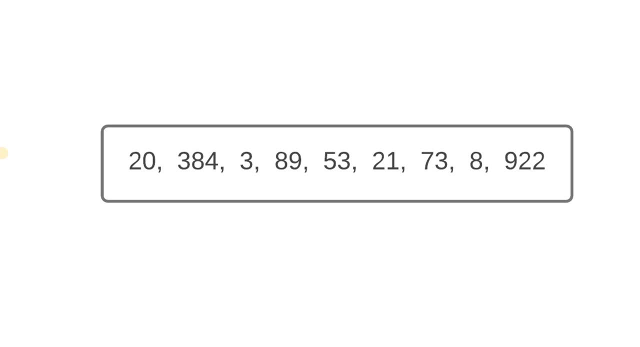 Radix Sort algorithm In the third one. in the third part, we'll take a look at how Radix Sort compares to other algorithms, and then we'll just generally talk a bit about Radix Sort and where it's used. Alright, so if you don't understand, 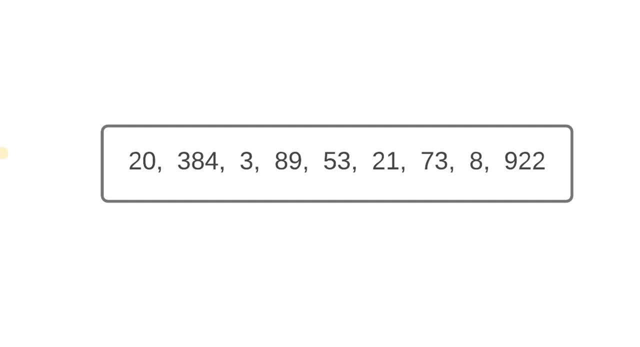 something in this part. alright, then wait for the coding part. alright, because some of the more technical details on how some things are being done is something we've already discussed in the coding part. alright, For now, just focus on how Radix Sort actually works, right, and its general concept. Okay, so notice over here. 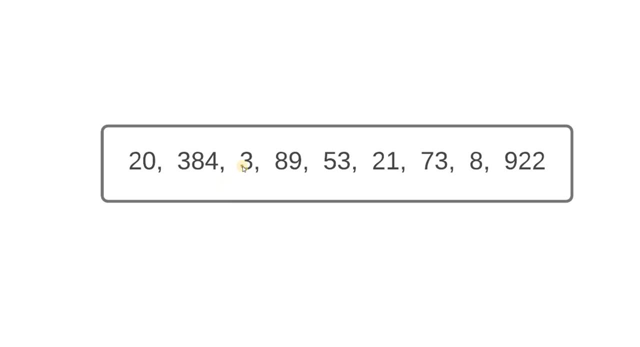 is that we have a wide range of numbers. Alright, We have single digit numbers, we have double digit and we have, you know, three-digit numbers as well. Okay, so Radix Sort. Radix Sort's basic concept is of using bucket and passes. 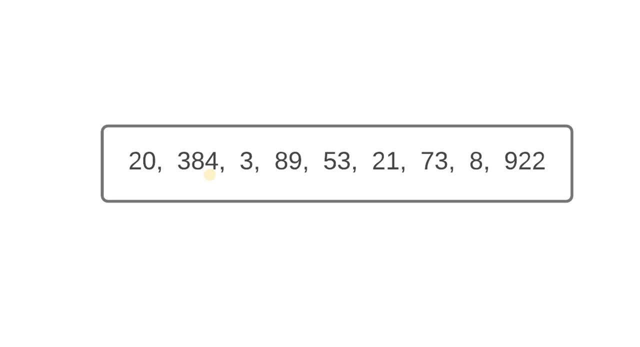 Now, what is a bucket? Well, imagine, Imagine a literal bucket as a slot. What we're going to do is create 10 buckets. Now, why 10 buckets in particular? Well, that's because there are 10 numbers, from 0 to 9.. 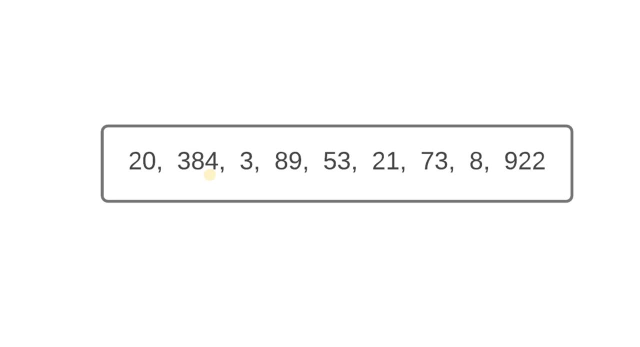 So we're going to create one bucket for each number And then we're going to put these numbers into these buckets after checking for a certain condition- More on that later. So RadixSort can actually also be used for strings. So in that case you would make 26 buckets. 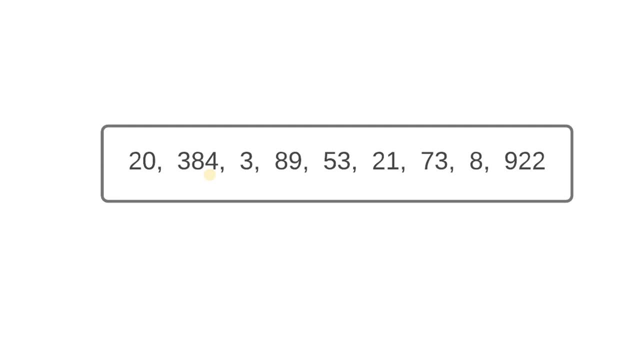 Because it's from A to Z. there are 26 characters, so you would make 26 buckets, But right now we're doing numbers, so it's 10 buckets. Another thing that you should know is that RadixSort makes passes. It makes passes based on the number of digits, of the highest number. 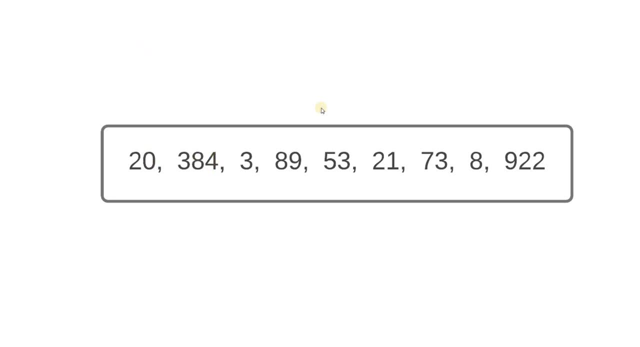 Now, what is the largest number? It's the largest number here Now: 20, no 384, no 21,, 273, no 8, no 922.. 922 is the largest number. So that's the first thing we do in the RadixSort algorithm. 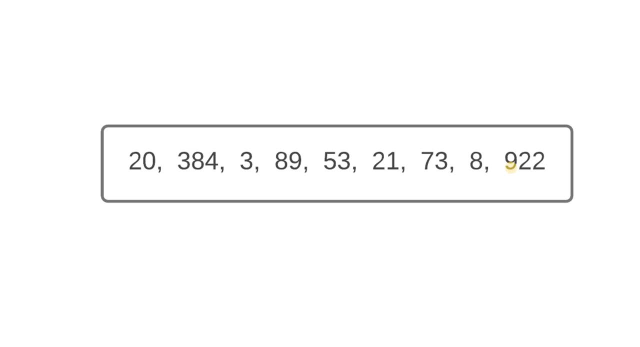 We locate the maximum value And then we check to see how many digits does it have. Well, 922 has 3 digits: 9,, 2, and 2. So it has 3 digits. So we're going to make 3 passes. 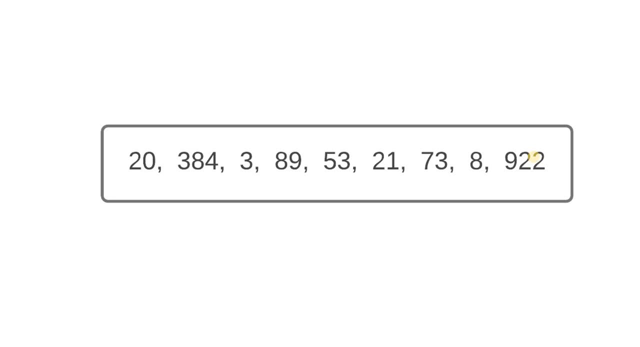 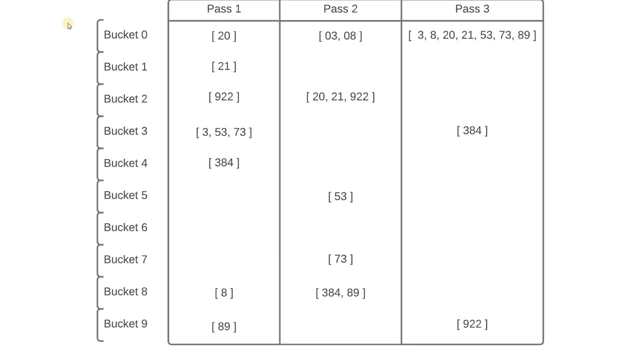 Now, what are we going to do in these passes? Don't worry, I'll explain that Now. let's actually move ahead to the next slide. All right, So here's our pass table. Now, this may seem like a whole lot to take in at once. 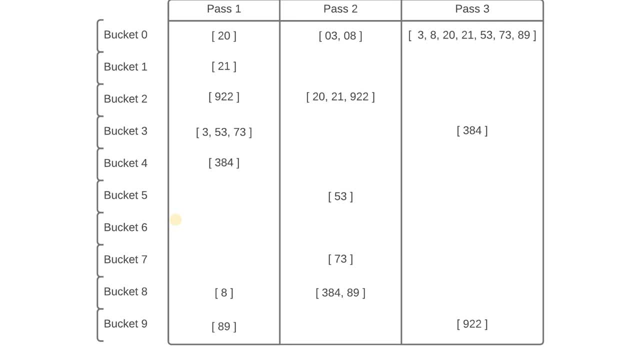 So just calm down and slowly take a look at it And let me explain things pass by pass, bucket by bucket. We're going to be on this slide for the next five minutes. All right, Stay calm, Stay calm. So pass 1.. 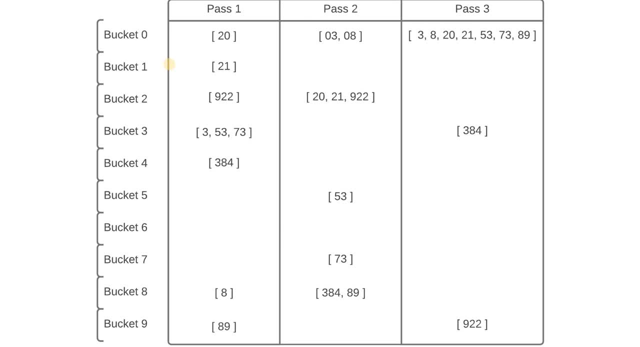 What we're going to do in pass 1 is sort. Well, not sort. All right, I don't want to use the word sort here, because we're not comparing and sorting. What we're going to do is place the values into the bucket based on the first digit. 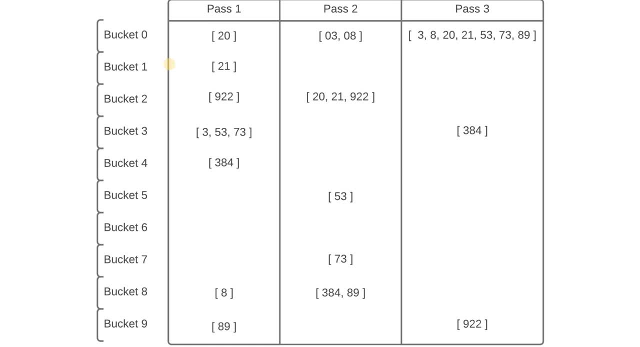 All, right, And the first digit I'm talking about from the right. Okay, So the you know the unit 10 and 100 digits. You know that system, we used to learn, So think of it that way. So we're going to be looking at the unit digit right now. 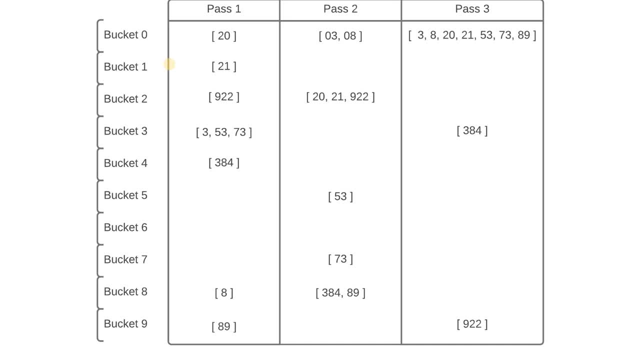 Okay, So we're going to be putting them into the buckets from 0 to 9.. All right, Based on this, you know this digit, the unit digit. All right, So let's actually begin sorting these values and putting them into the correct buckets. 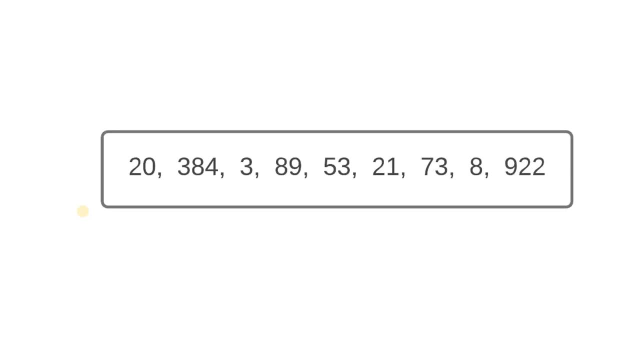 and doing all three passes, Let's come back to this slide. All right, This slide shows the original list of numbers. Okay, So number 20.. That's the first number that we're going to be dealing with Now. what we're going to do is locate the correct bucket to put this into. 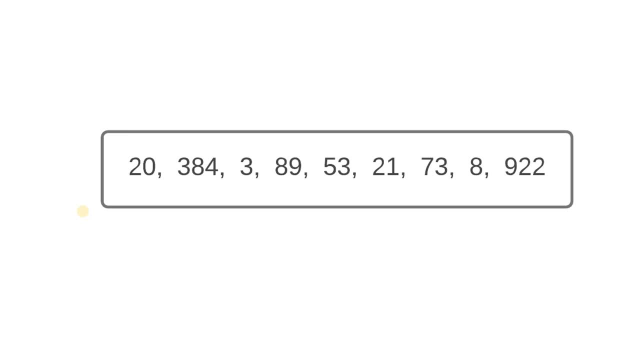 Now we do this again. as I mentioned earlier, we do this based on the unit digit, All right, And in this case, the unit digit is 0,, which means that we're going to put this number into bucket 0.. 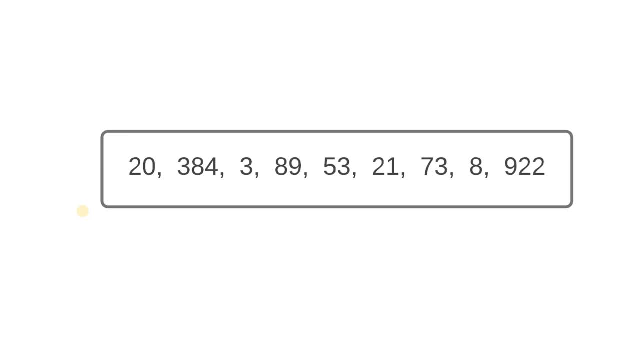 All right, Now we'll cover this mostly in the code section, But I'll just briefly describe here how to actually, you know, locate this unit digit. All right, How to find 0.. All right, These aren't strings. 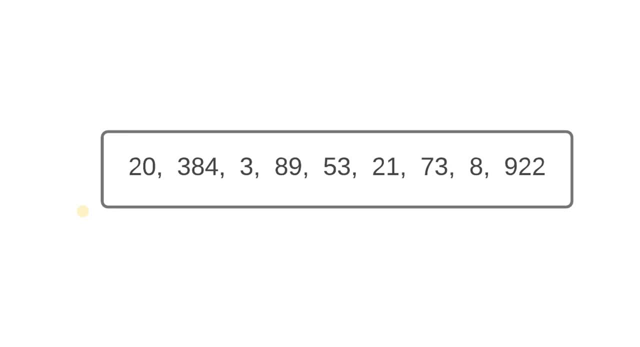 So you can't use string indexing here or anything, All right. But a very easy way of doing this is using the mod and floor division, All right. So in this case, all you have to do is mod 20 by 10.. 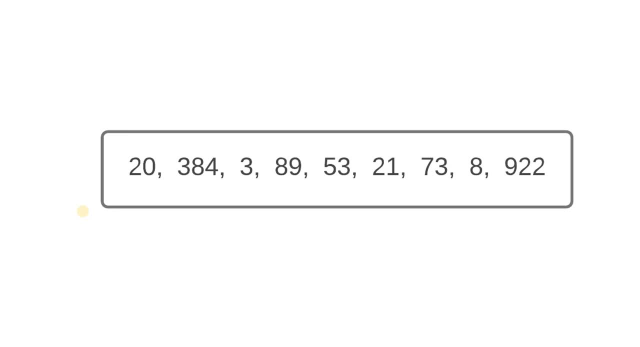 Okay. So if you don't know what modulus is, modulus returns the remainder, Okay. So if you divide 3 by 2, okay, the modulus will return 1.. Because that's what gets left over, right when you divide 3 by 2.. 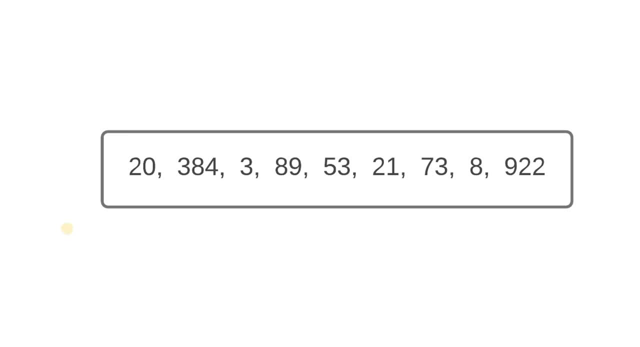 Okay, So in this case, 20 mod 10 gives 0.. All right, It's a clean division, All right. 20 divided by 10 gives 2.. All right, There's no fraction involved. All right, So in this case, 20 mod 10 gives 0.. 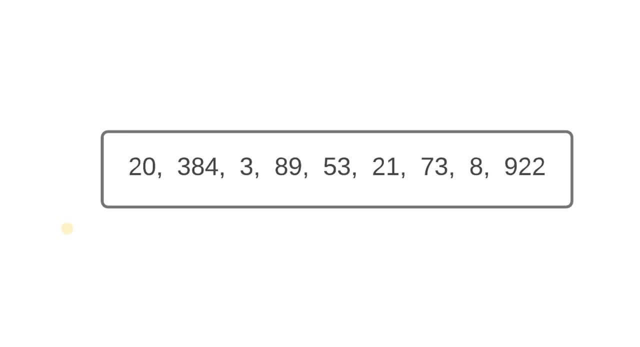 So we'll use this return value 0 to put it into the correct bucket, Bucket 0.. So our code looks something like index, where index is a variable, Index is equal to 20 mod 10.. It's a bit more complicated than that, but we'll get more into that later. 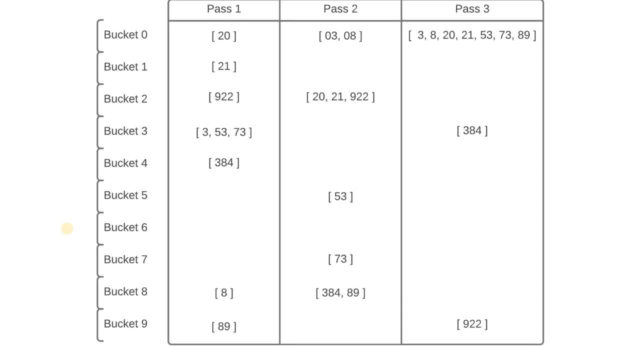 Okay, So yeah, Now you can see clearly in this pass table that 20, the value of 20 over here, okay, at the very top, is in bucket 0.. Okay, So next is 384.. Now let's mod this by 10.. 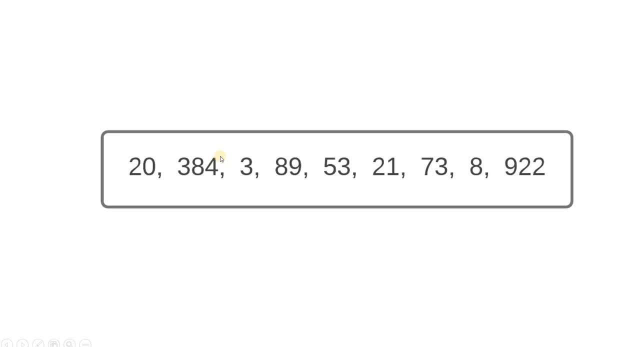 What do we get? We get 4.. All right, Because of this value, And let's put that into bucket 4.. Okay, We can see that over here. It's in bucket 4.. Next is 3.. This is again very simple. 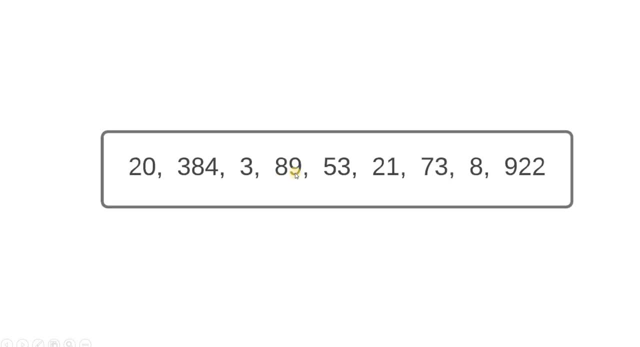 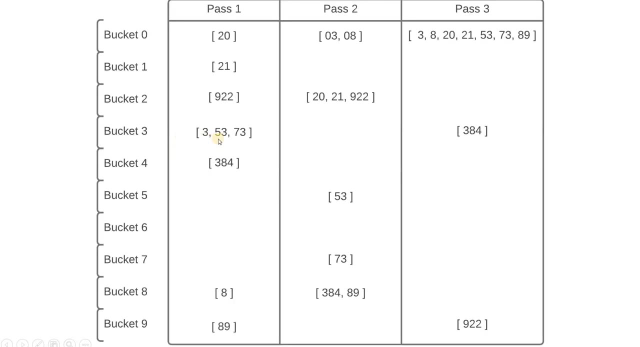 It'll go into bucket 3.. Okay, You can see that over there. The value 89, it goes into the ninth bucket. Okay, Then the value 53, it goes into the third bucket again. Okay, And remember Each bucket is its own list. 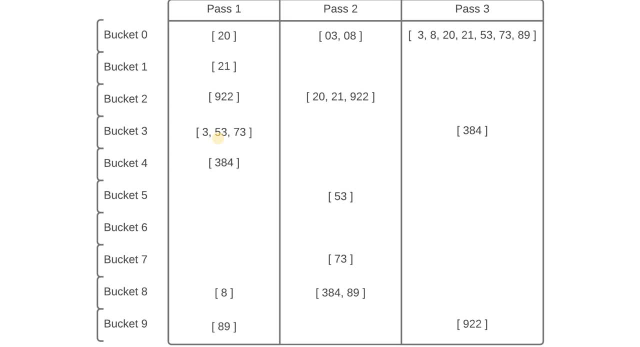 It's a separate list, So we're just appending onto that list. So basically, we have a 2D list here. Okay, It's a 2D list that has 10 lists within it And, of course, each list is the bucket. 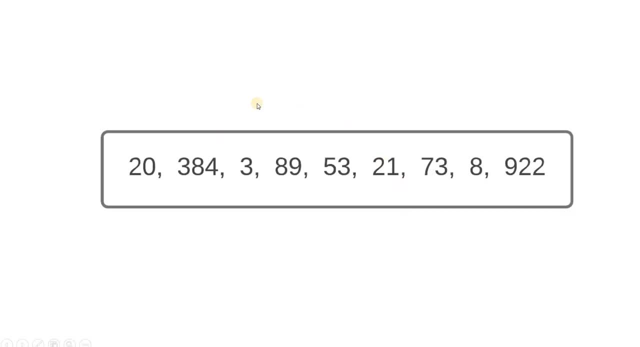 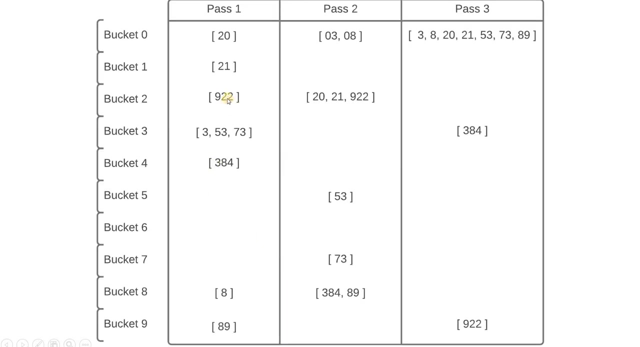 Okay, All right. So 21 goes into the first bucket, 73 goes into the third bucket again And 8 goes into bucket 8.. And over here this value- 922, goes into the second bucket. So that's the first pass complete. 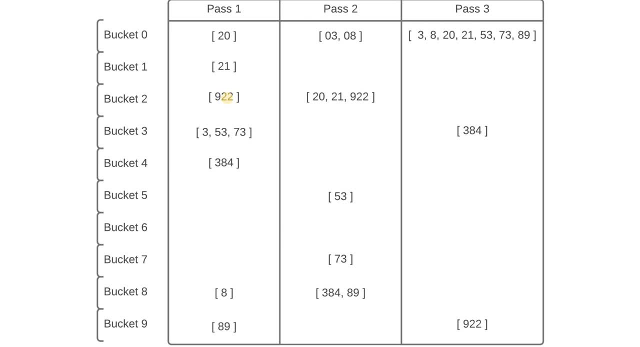 Now I want you to notice something rather interesting. If you just look at the first digits, the unit digits of each number, you'll notice that we have a perfectly sorted array. Watch Over here. Over here you can see 0,, 1,, 2,, 3,, 4.. 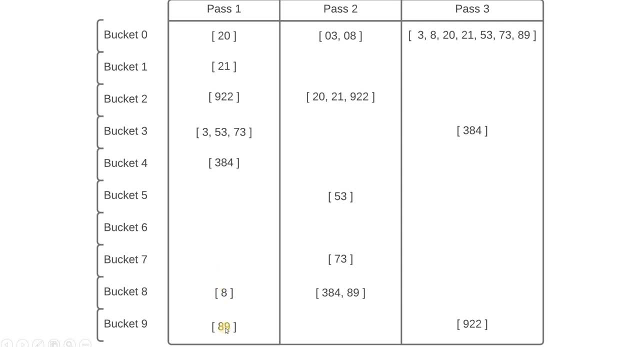 And there's nothing over here, of course. So 5,, 6,, 7,, 8, and 9.. Now, just keep that in mind. This will make more sense in the next pass. Okay, So we're on pass 2 now. 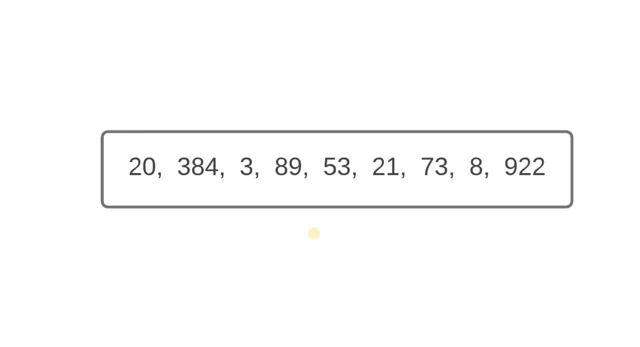 All right. Now here's a slight change. Well, the change is mostly in the code, so you won't notice that here, But basically we now need to look at that digit 10.. You know the digit at the 10th place. 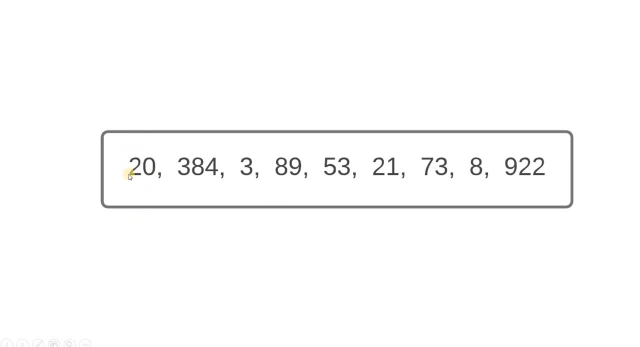 So basically 20 over here. All right, We look at 2.. Okay, We get the value 2. And then we put it into bucket 2.. Now again, I'll give you a brief intro on how we're actually going to do this in the code. 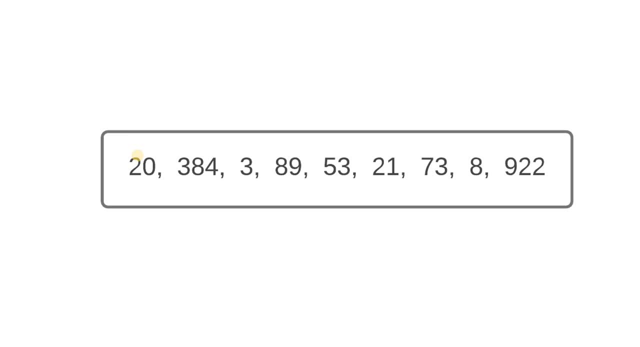 So what we do is floor division. All right, Basically, we divide 20 by 10.. Okay, So 10 is actually to the power digit, Okay, Where the digits actually start from 0. So again, if you don't understand this right now, that's fine. 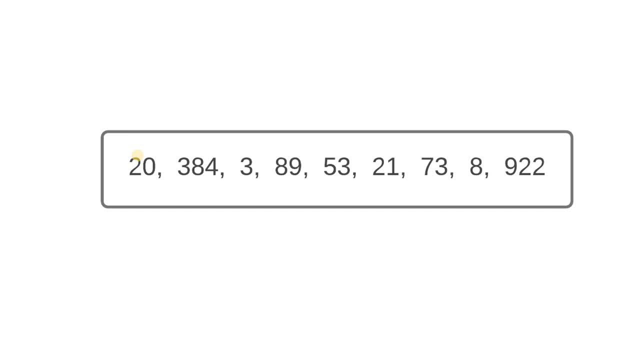 All right, I'll explain this again in the code section. So we do 10 to the power digit. Okay, Where digit starts from 0. So in this case we have 3 digits in total. All right, 3 max digits. 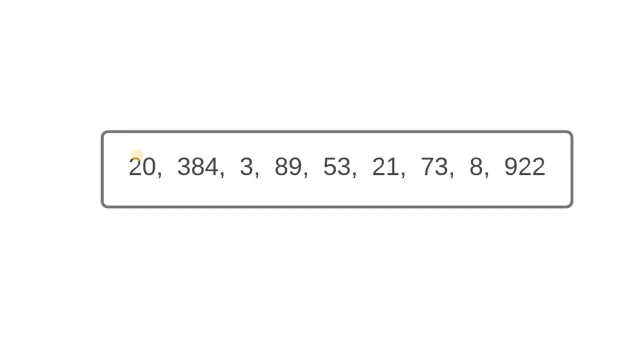 So we do 0,, 1, and 2.. Now in the first pass, 10 to the power digit, 10 to the power, 0 is 1.. So that's why the division didn't show Okay. So we just cleanly divided- sorry, modded- 20 by 10.. 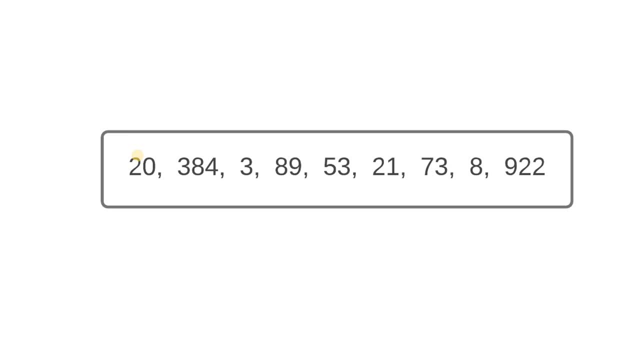 All right, So the code was actually: index is equal to 20 divided by 10 to the power digit modded by 10.. Okay, Now again, I told you because the digit was to the power 0.. Okay, We didn't notice it in the first pass. 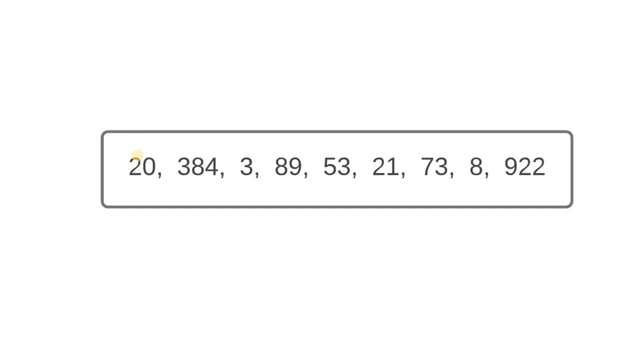 But now we're basically in the second and third pass. this actually makes a difference. So what we're going to do is first divide 20 by 10, which gives us 2.. And then we'll mod this by 10, which gives us 2 again, which makes it go into the second bucket. 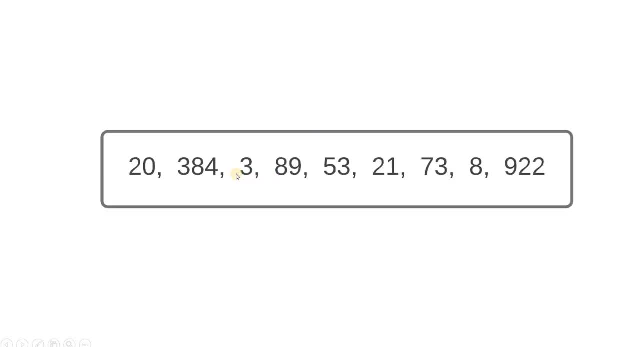 And there you go: 20 is over there. Okay, Now let's take a look at this one: 384.. Now I mentioned the term floor division once or twice. So what floor division basically? is that if you divide a number like 384, okay, if you divide this by 10, we'll get 38.4, right? 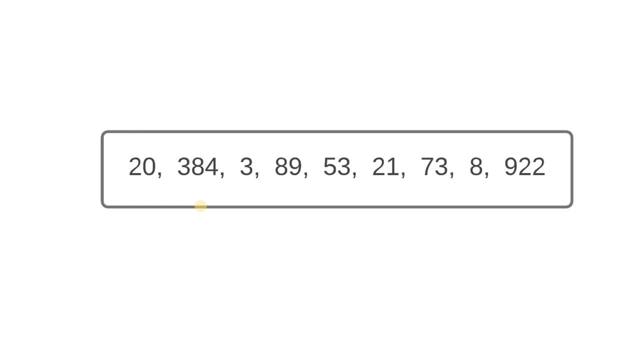 What floor division does basically is it removes the fractional part. So, instead of giving us 38.4, it gives us 2.. So, instead of giving us 38.4, it gives us 38.. All right, Then we'll then mod 38 by 10.. 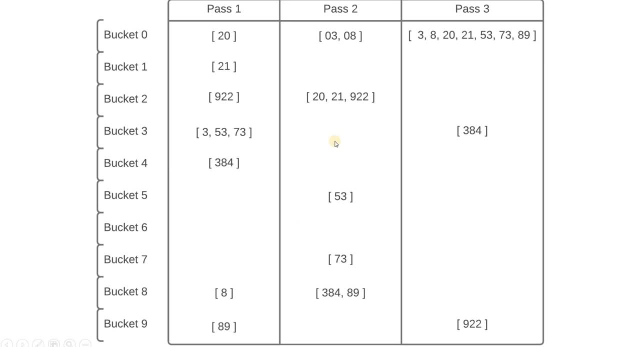 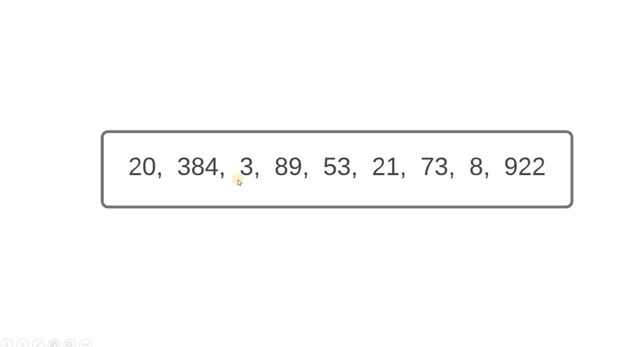 And then we'll get 8.. All right, Pretty simple and straightforward. This goes into the eighth bucket. All right, Right here, And here's 3. now, Again, there's no need to complicate this. One useful trick that you can, you know, use when you're dealing with second and third passes on small numbers. 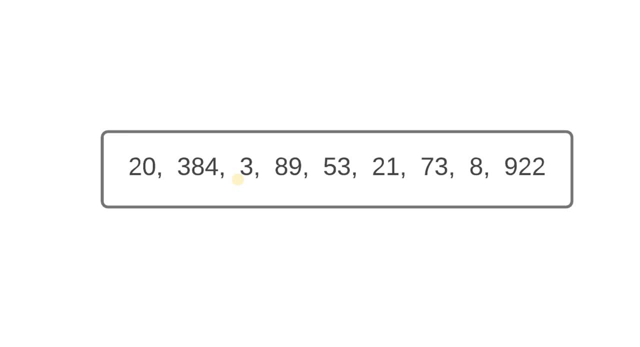 Like the left and the right, Like 3 over here. It's a single digit, So you might think of it. and how are we going to divide this by 10 and stuff? You don't need to actually think that hard on it. 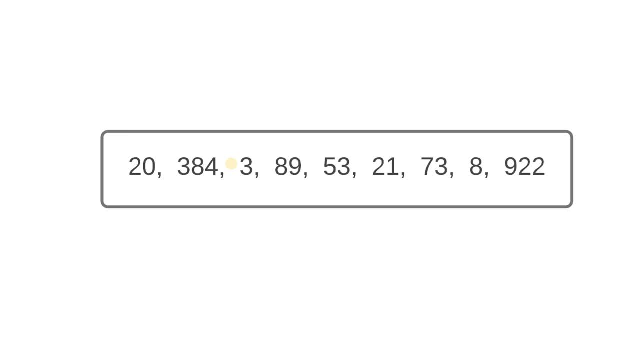 Imagine that there's zeros. All right, Imagine that there's some extra zeros over there. Imagine that instead of 3, it's actually 003.. Okay, You can sort of imagine all of these as the three-digit numbers, But you know there's a zero over there. 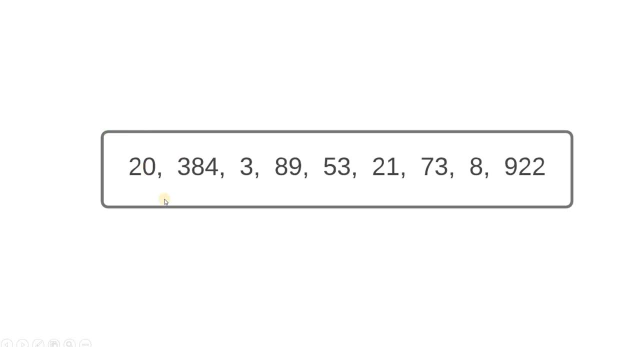 Like 020.. It doesn't make an effect on the actual number, It's just there to sort of help with your concept, if you find that it makes it easy to understand. So yeah, 3 divided by 10 is equal to 0.3.. 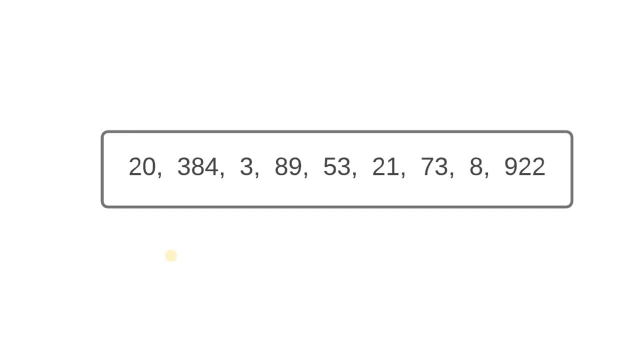 But since we're doing floor division, it's equal to 0. And then 0 mod 10 is equal to 0. So we put that in bucket 0. And then there's 89 over here. It's the same thing. 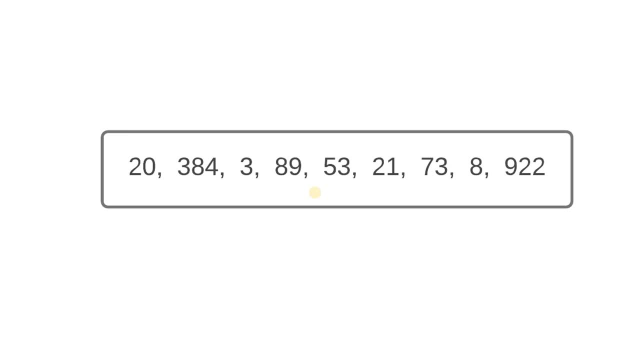 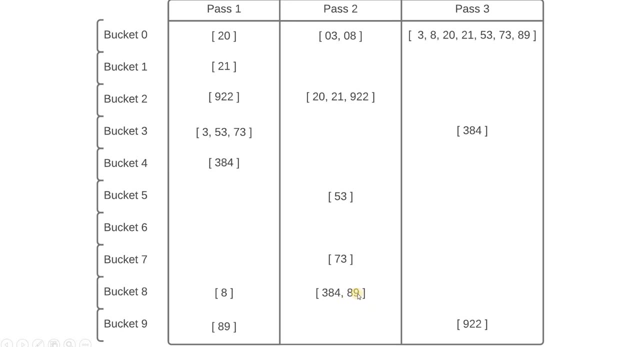 We divide it by 10.. We get 8 modded by 10. And we get 8.. So we put it in the bucket 8.. So you can see it in bucket 8 over here. 89.. Okay, And 384 was already there. 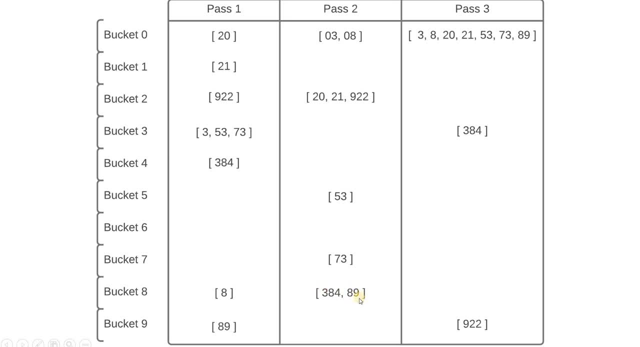 All right, So that's why 89 gets appended after it. Okay, And you can look at bucket 0 over here. There's 3 over there. It's not actually 03.. It's just 3.. I just put the 0 over there just so that you could sort of visualize it. 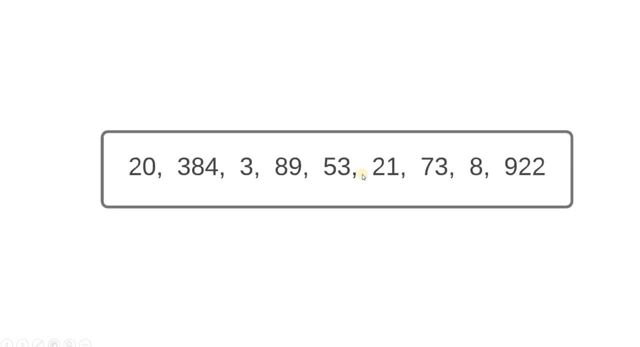 All right, Okay, So back here Now. 53,, 21,, 73,, 8.. They're all done in the same manner, All right. So we need to repeat that. Let's take a look at 922.. So we'll divide that by 10.. 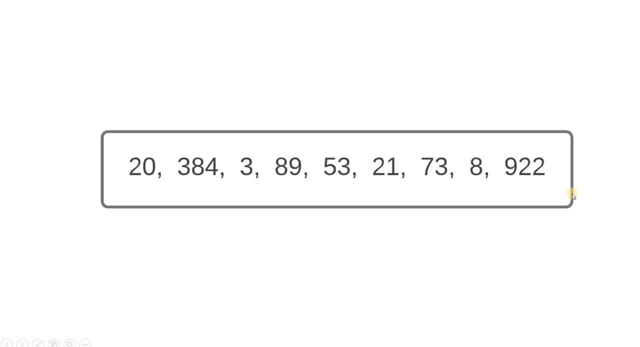 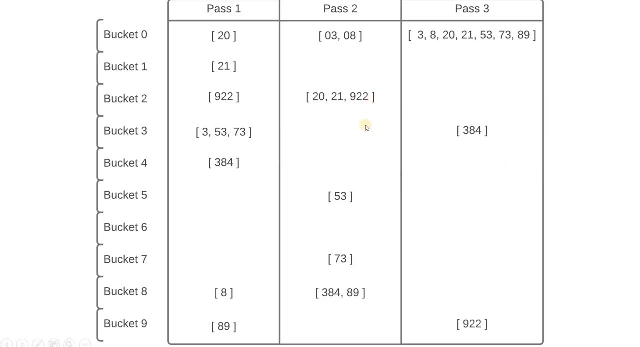 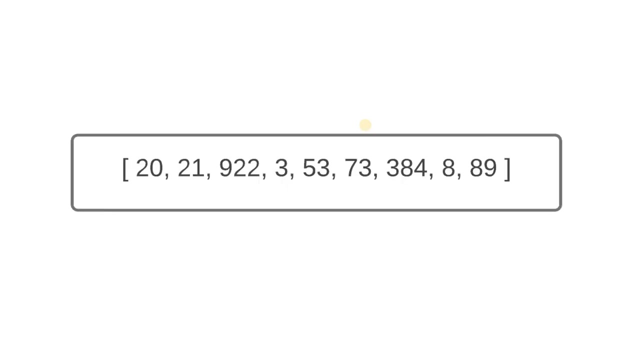 We'll get 92.2 rounded off- I'm sorry, Floor division. So we get 92 modded by 10. We get 2. Okay, And then we put that here in bucket 2. Okay. So now let's take a look at something a little further ahead. 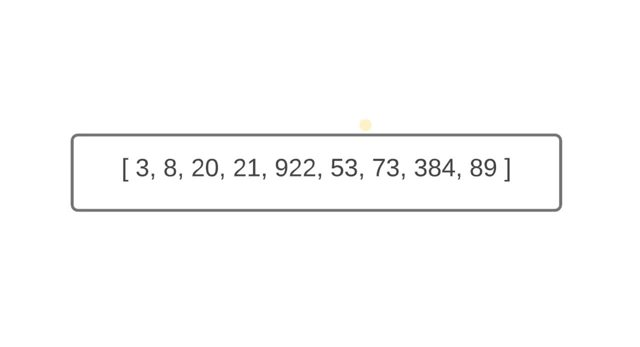 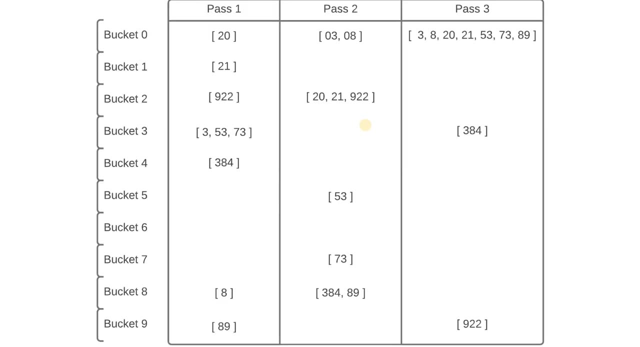 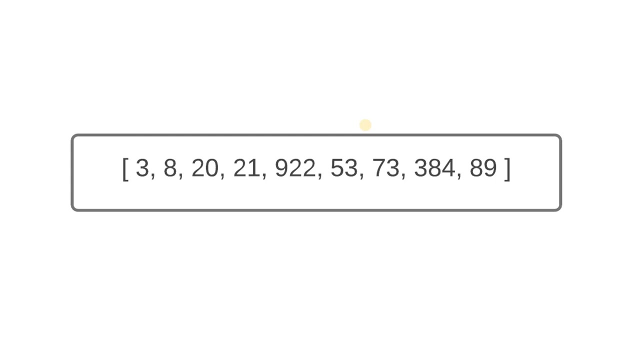 Okay. So this is what the array looks like At pass number 2.. Okay, If you were to sort of take all the buckets in pass 2 and append them together, Okay, You would basically get this. I want you to notice something now. 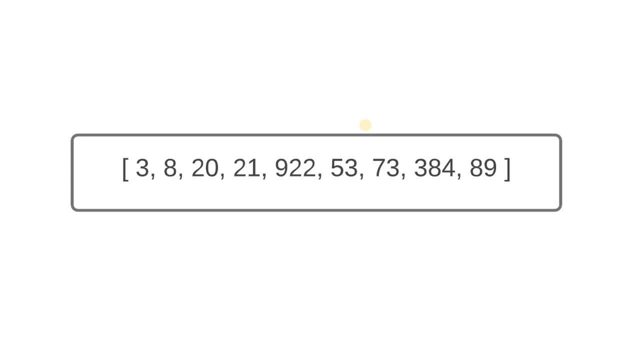 If you were to remove the 2, 3 digit numbers, we have a perfectly sorted array. You see that. So, basically, what's really happening is that the first pass sorts all of the numbers, Sorts all of the numbers based on the first digit. 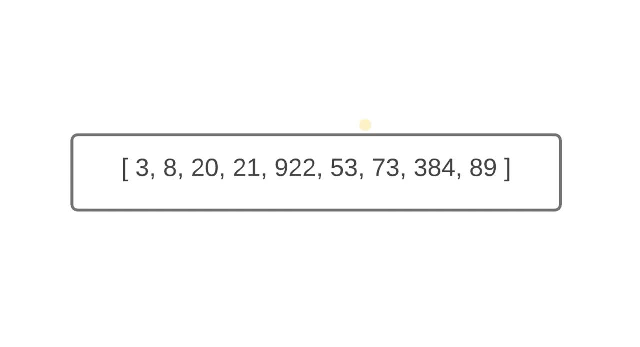 So, basically, every single digit number in the first pass will become sorted. All right, It will be in its correct position relative to each other. In the second pass, all the 2 digit numbers and the first digit numbers will become sorted, And in the third pass we'll sort all numbers. 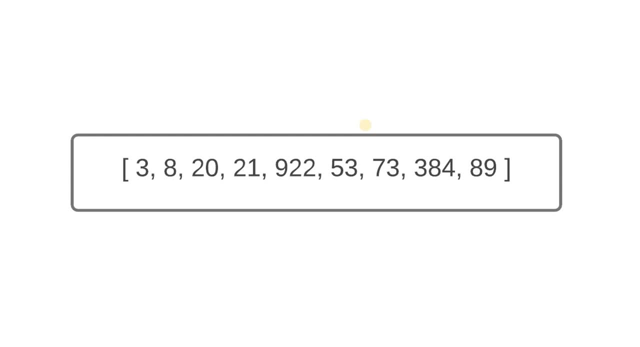 The single digit ones, the double digit ones and the 3 digit ones. Okay, So in the third pass, these 922 over here and the 384 over there will become properly sorted, All right. So, yeah, Let's get back into the pass table. 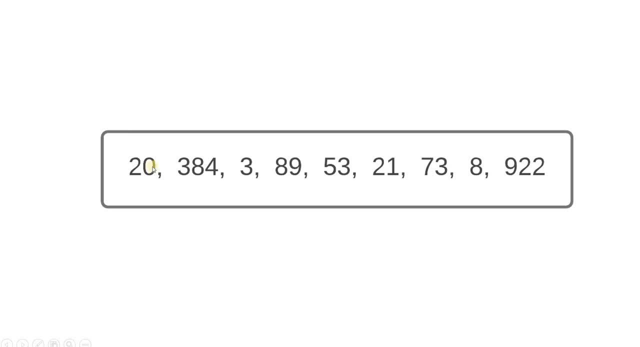 Okay, So let's move on to the third pass now. So 20 over here, Basically. now we're going to increase the division operator. Previously we were dividing by 10 to the power 1.. Now we're going to divide by 10 to the power 2.. 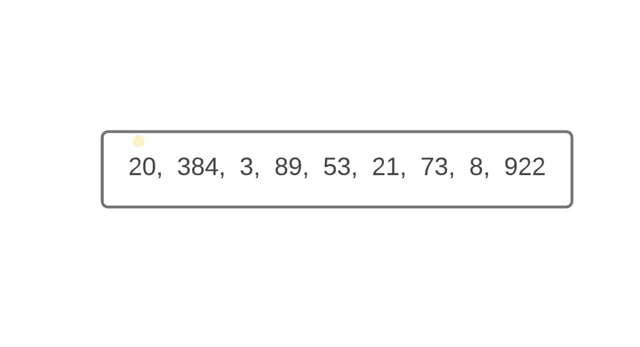 Okay, So it's 20 divided by 100, which gives us 0.. And, of course, modded by 10, that gives us 0.. Okay, And this is going to be the case for anything. that's not a 3 digit number. 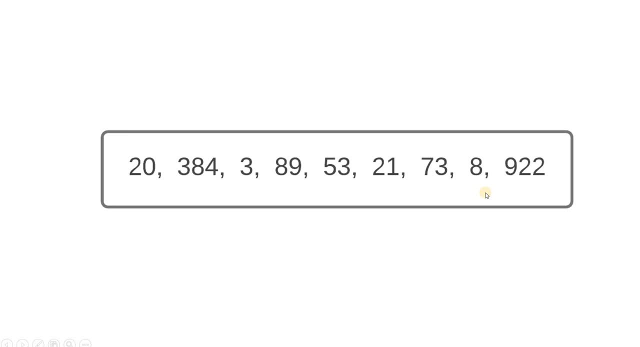 23,, 89,, 53,, 21,, 73, 8.. They're all going to go into the bucket 0.. Because you divide them by 100, they all give 0.. All right, Floor division. Let's take a look at 384 and 922.. 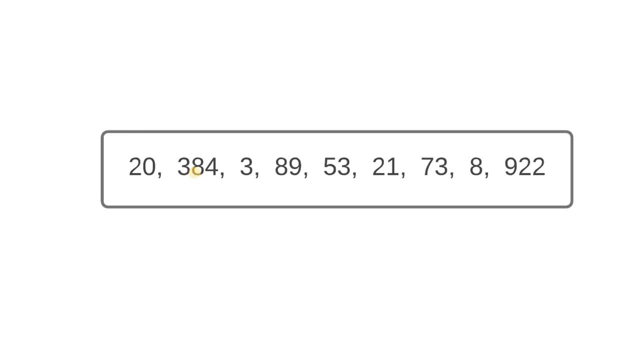 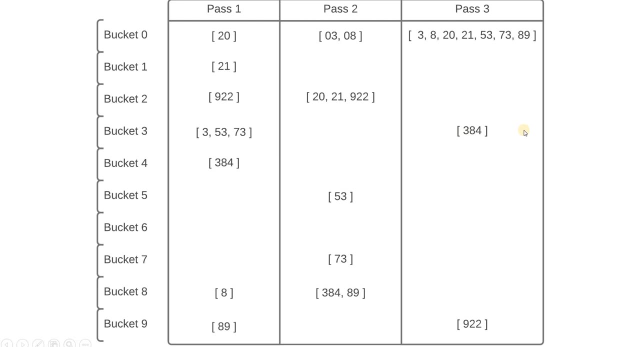 So 384.. Divide that by 100 and you get 3.84.. Floor division: So you get 3.. Modded by 3.. Sorry, Modded by 10. You get 3.. It goes into bucket 3.. 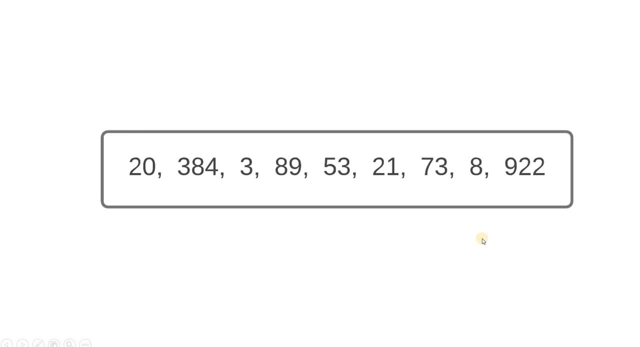 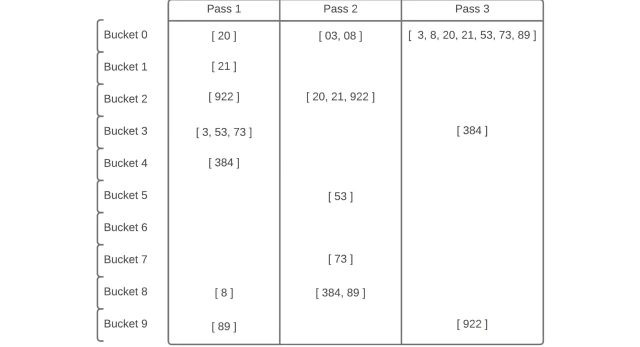 922.. Divide that by 100.. You get 9.22.. Floor division: You get 9.. Modded by 10. You get 9, which makes it go into bucket 9.. Okay, So now let's properly take a look over here. 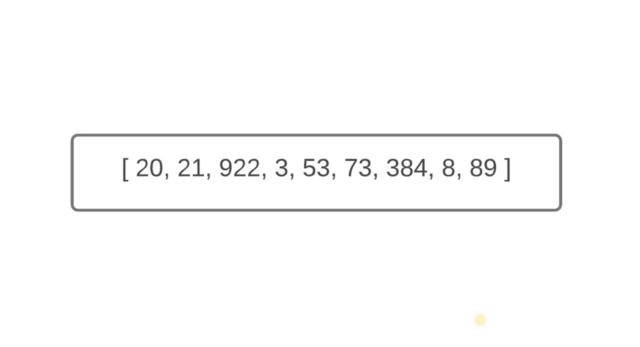 This is what it looks like in the first pass. Okay, Again, not much to look at over here. This is what it looks like in the second pass And this is what it looks like in the third pass. Okay, So now we're done here, basically. 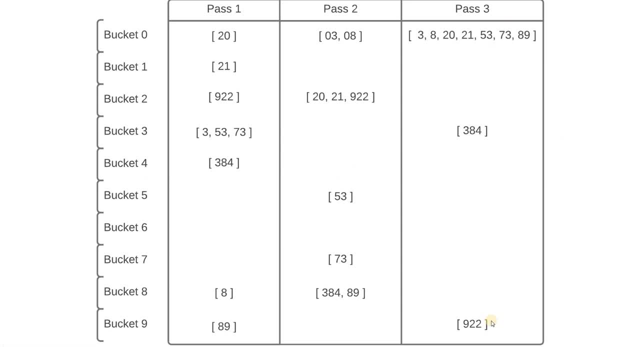 Now let's just go back here and I want to show you over here, basically, that we're basically going to add together these three lists. Okay, We're going to add bucket 0, add bucket 3, add bucket 9.. But we're actually going to be adding all of them. 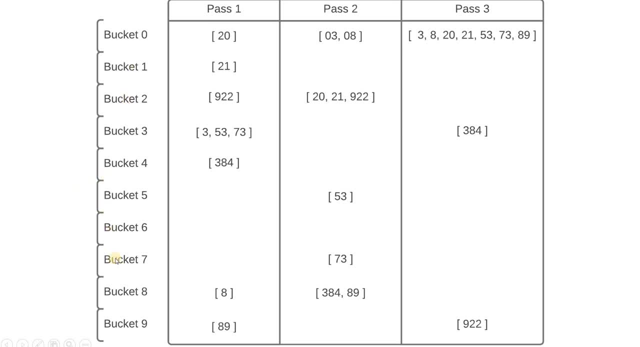 Right, But since there's nothing in bucket 1,, bucket 2,, bucket 4, bucket 5, bucket 6, bucket 7, bucket 8, it won't make a difference. Okay, So now we're done with the visual representation part. 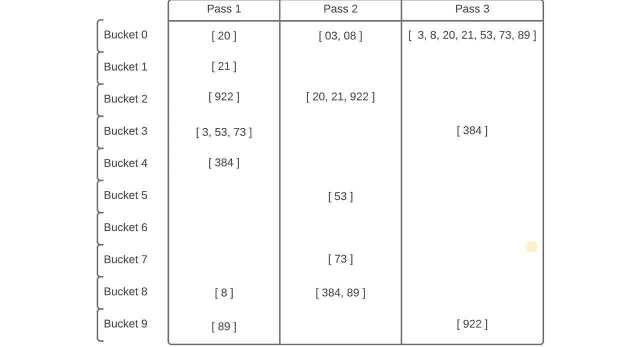 Okay, So let's actually get to the code part. Okay, Because there's still one step that I can't actually explain over here, And the step has something to do with flattening- Flattening the 2D list into a 1D list. 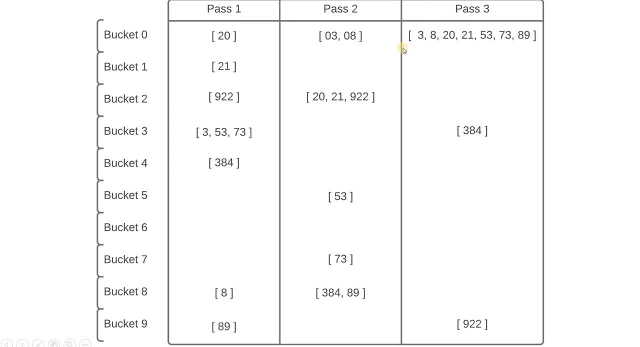 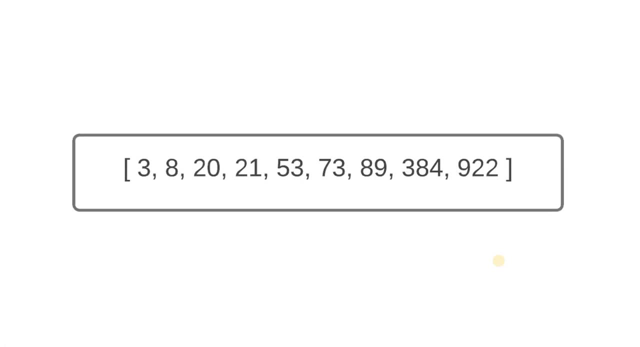 Because this is still a 2D list. All right, These are three separate lists. This is not one list. Okay, The stuff I'll show you over here. this is just for visualization purposes. Okay, So that's the one step left that I'll take a look at in the coding section. 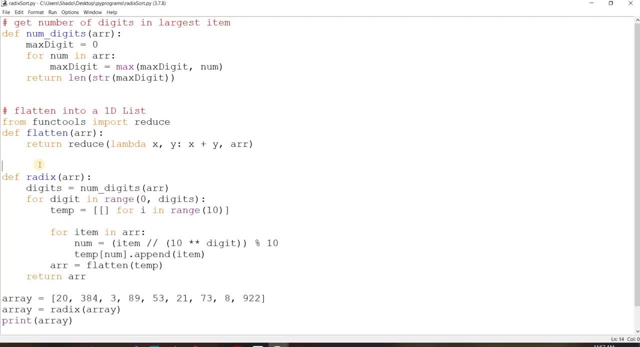 All right, So let's move on to that. All right. So here we have three functions. The main logic of periodic sort is in here, But the other two are utility functions that help us during the process. So this one is pretty simple and there's no need to explain it too much. 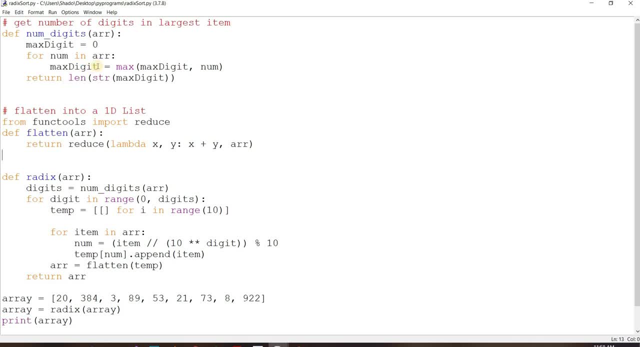 But basically what it does is that it finds the maximum digit, All right, And then it stores it in max digit And then we convert it to a string And then we find out the length. So what this basically does is returns the number of digits in the graph. 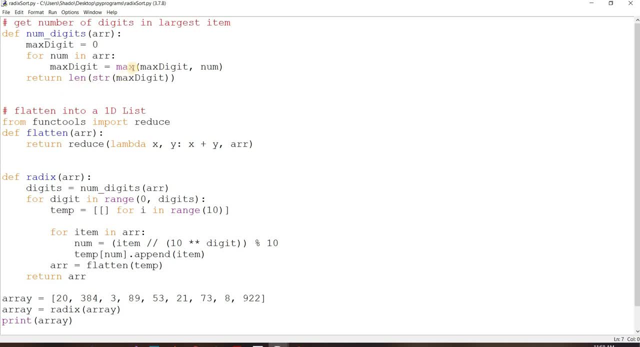 And it's in the greatest number. Okay, And we did this using the max function. All right, It's an inbuilt function in Python. All right, Finds the maximum value. Okay, So here is the list, flattening More on this later. 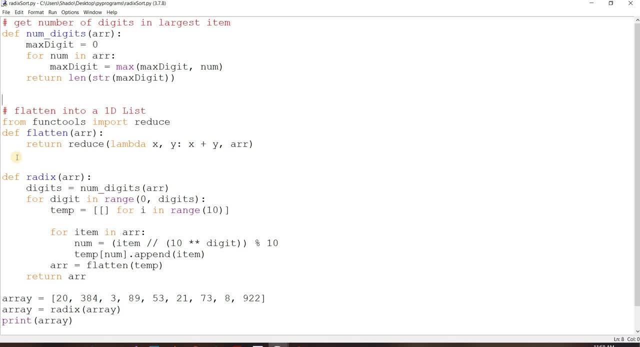 But it's used to actually combine the lists, All right, And from 2D into 1D. What it basically does is combines all those 1D lists In the 2D list Into 1.. All right, That's what it does. 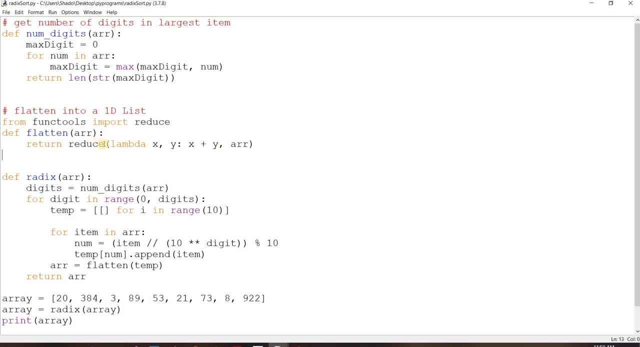 So that's what the plus here is actually about. Okay, It's just. you know, it's an inbuilt function, It's part of the func tools library, You just need to use it. All right, Like this. I'll also make a video on, you know, flattening 2D lists into 1D lists. 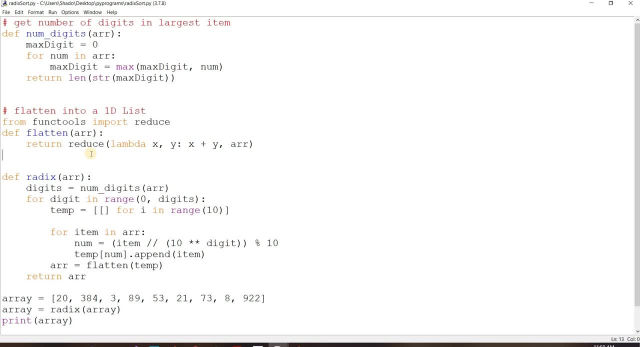 Because there are actually like four or five ways. You can even make your own. You can use list comprehension, You can use reduce, You can use sum as well, So let's just move on to the RAIDX function now. All right, 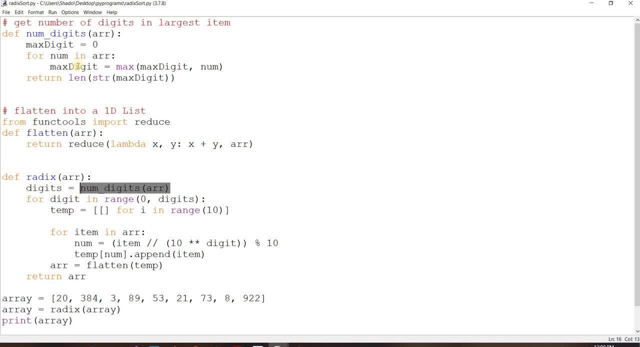 This is the main part. So over here we call numDigits, Okay, And then we store the digits in digits And then we set up this for loop. This is the for loop responsible for the passes. Okay, So the largest digit here is 922.. 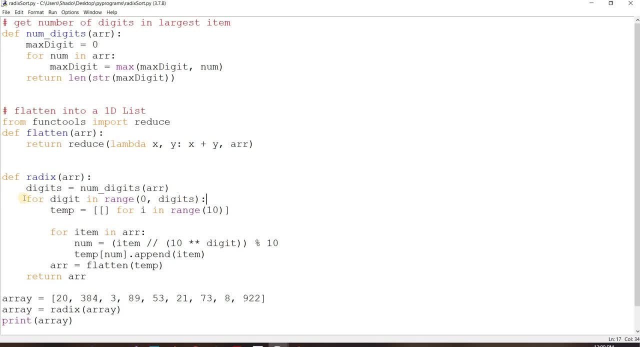 And it has three digits. So we run the for loop from 0 to 2.. And that's what I meant earlier When I was talking about like 10 to the power 0,, 10 to the power 1,, 10 to the power 2.. 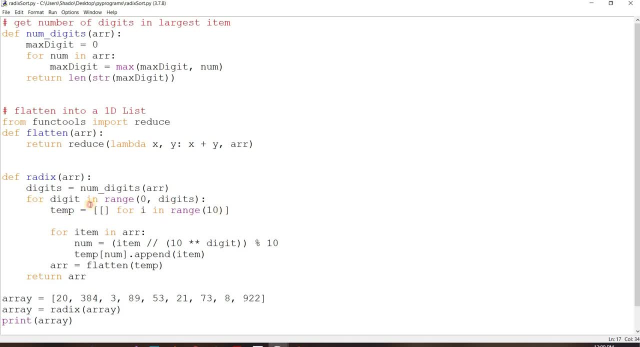 This is what I meant. Okay, So this is where we create the buckets. Okay, You can just call this buckets, if you wanted to. I just call it temp, because it's just a temporary array that you'll recreate each time, You know, in each pass. 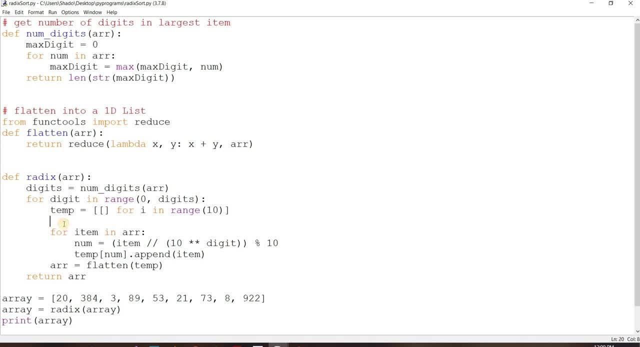 Okay, And over here we iterate over the array. now, Okay, And what we do is num. This is basically the index. You can also think of this as index. Okay, So we do. index is equal to item, which is the value. 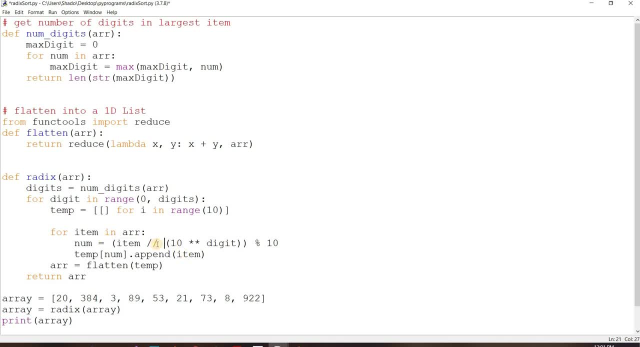 For example, 20.. Okay, So we floor divide this. This is the symbol for floor division. This is division. This is floor division. All right, That's it. So here we divide it by 10.. Since this is 20, we're talking about. 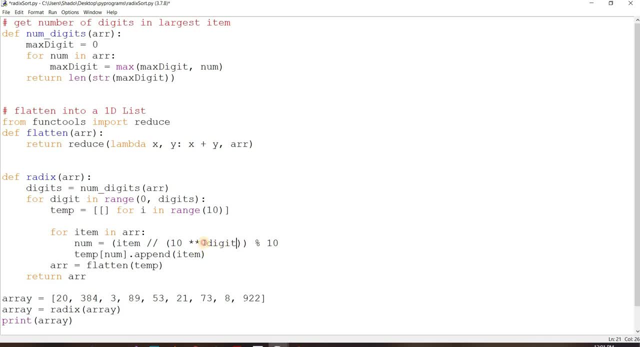 And in the first pass. So it will be 0.. Okay, Digit will be 0 because of this. over here It starts from 0. Mod 10.. So 20 divided by 10, which is 2. Mod 10,, which is. 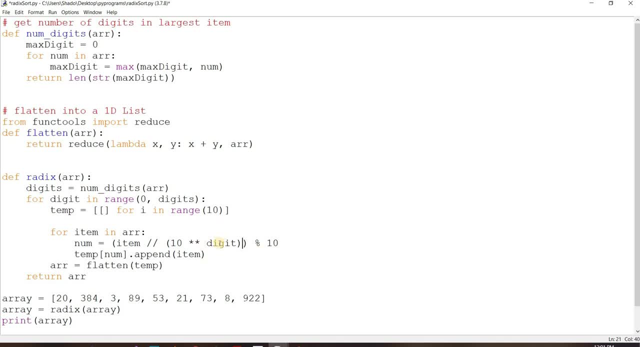 Okay, Hold on. Sorry, Sorry. This is the first pass, Right. So digit will be 0, which means 20 divided by 1.. All right, 10 to the power of 0 is 1.. So 20 mod 10 is 2.. 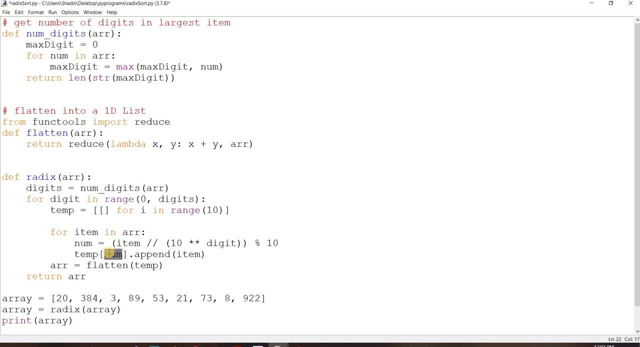 And then temp 2.. So basically it's like this: Temp 2.. This is the index number 2 of the 2D list, temp, which means bucket 2.. You can also think of it as bucket 3, because we start from 0.. 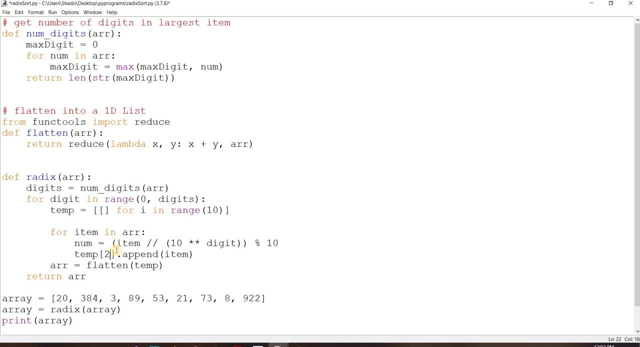 Right: Bucket 0.. Bucket 1.. Bucket 2.. So don't get confused. I've actually maintained the notation from 0 from the start, So I'll just use that When I say bucket 2, it's bucket index 2.. 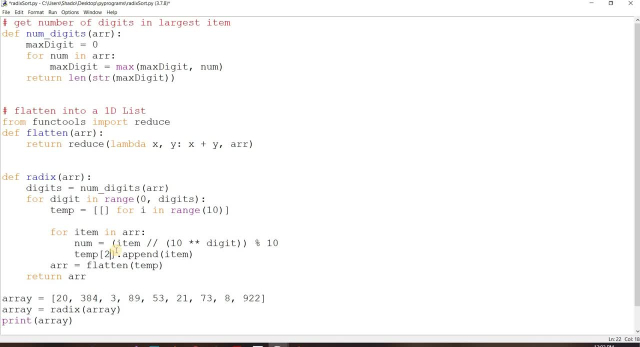 Okay, It's not bucket number 3, literally Okay, So yeah, And of course we just append this to that index, All right. Or to that bucket We append that value, All right. So we do this for all the values in the array. 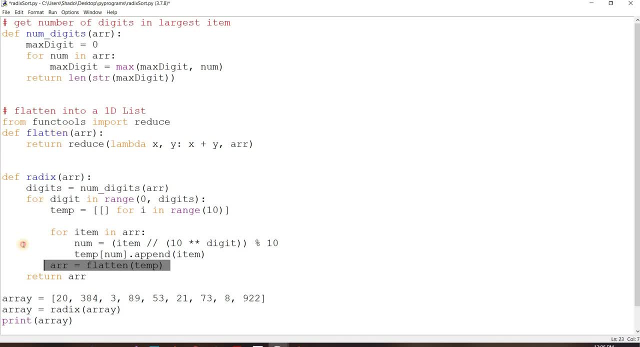 And then we flatten it. We call the flatten function. So basically what this does is that all the different lists- okay- that were created in the temporary array, it flattens all of them into a 1D list And puts it into array as the new array. 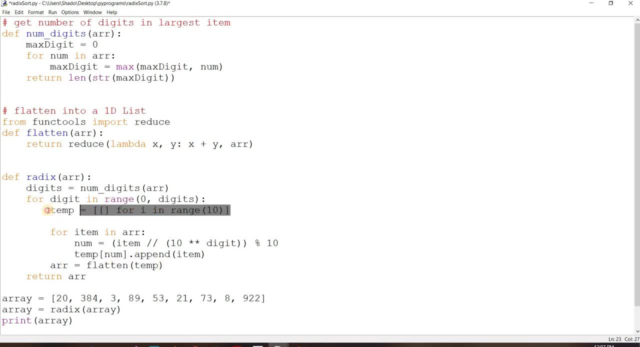 Okay. So then this repeats again in the second pass. We come over here, We recreate the bucket, I iterate over each value again, But this time with digit is equal to 1.. So, and you know, I explained all this earlier. 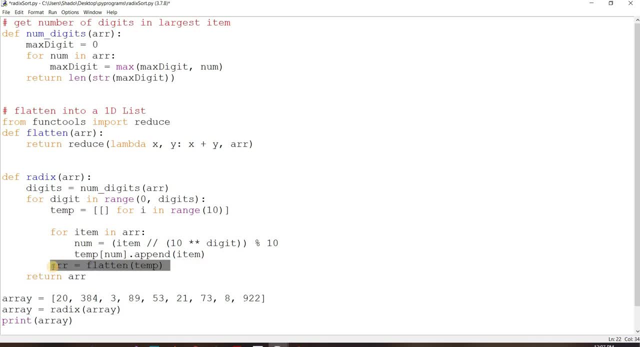 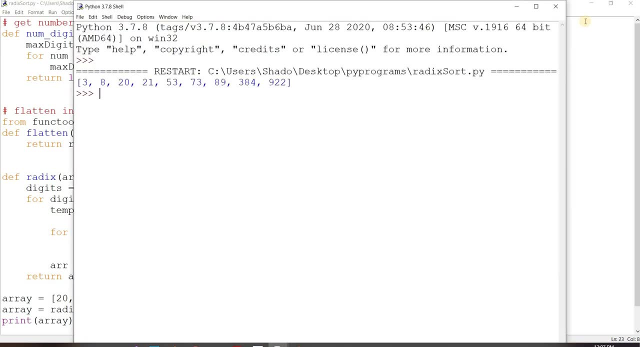 So we do this three times And by the end of it we have a fully formed array. Okay, So let's just run this once. Okay, There you go. You can see that right there And, if possible, there's something I want to show you. 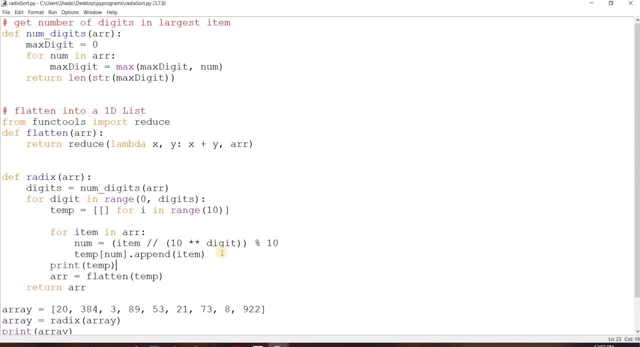 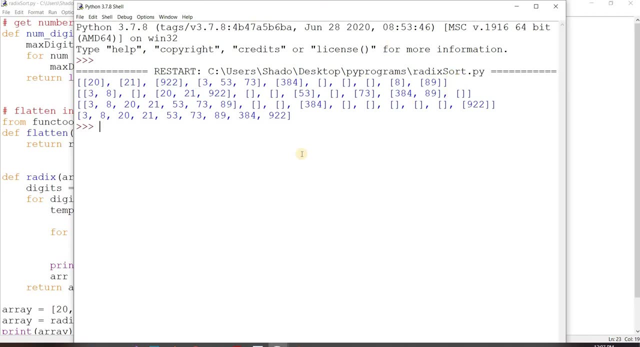 I want to show you what it looks like. I want to show you what temp looks like. Okay, There you go. This is pretty handy. I think This will probably help improve your concepts. You can also cross-reference this against the pass table I showed you earlier. 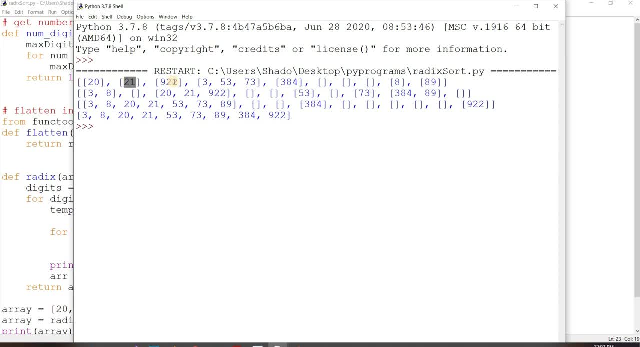 So you can see over here that this is the bucket 0.. This is bucket 1.. This is bucket 2. Bucket, 3. Bucket, 4. Bucket, 5. Bucket, 6. Bucket, 7. Bucket 8.. All right. 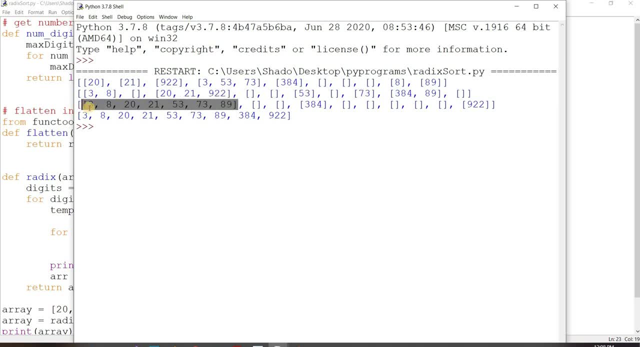 You can see they're all sorted accordingly And remember the third pass, where all of them were stored in the first bucket because the hundredth digit on each one of these is 0. And then this is stored in the third bucket because it's 3 over there. 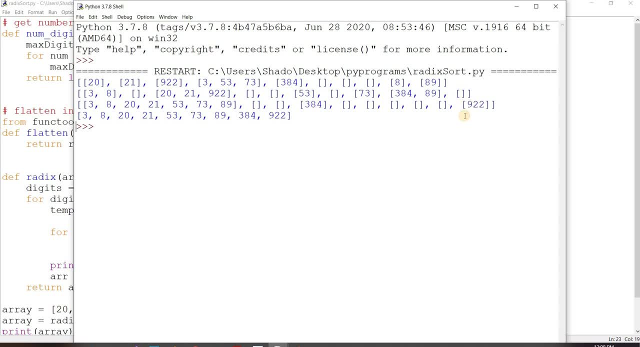 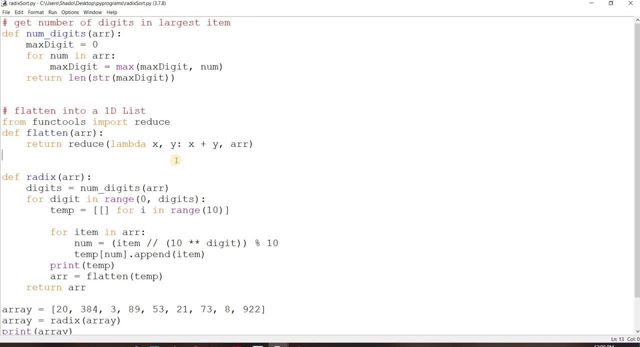 That's 9.. So it's stored in the last bucket, bucket 10, or bucket 9,, depending on which way you want to see it. So yeah, That's about it for the code. I mean, I don't think there's anything left to explain. 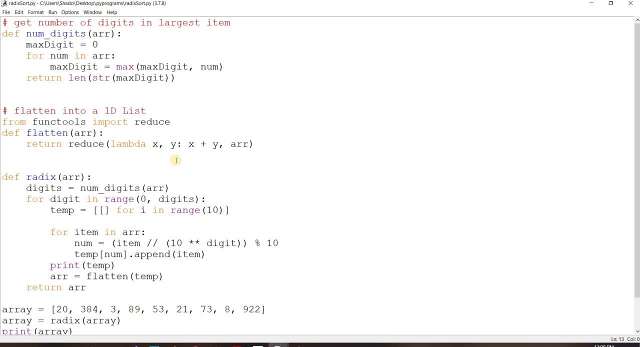 So let's just briefly discuss radix sort, now You know, as a sorting algorithm, and compare it to the others. All right. So one thing about radix sort is that it is really really fast for numbers, All right, And if you're trying to sort a very large list of numbers, radix sort is a great choice. 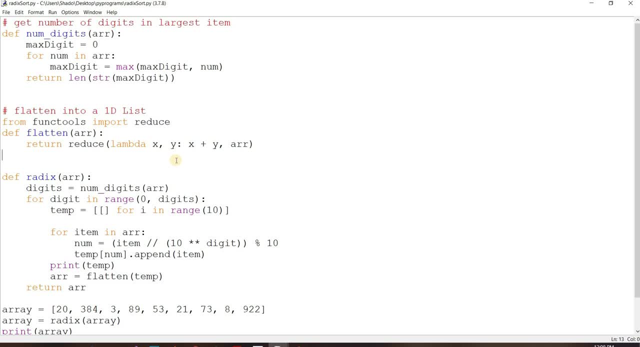 I believe there have been comparisons where radix sort is like three or four times faster than other sorting algorithms like quicksort. So yeah, That's really something especially for small numbers. By small numbers I mean digits like single or double digits, for instance, or even triple. 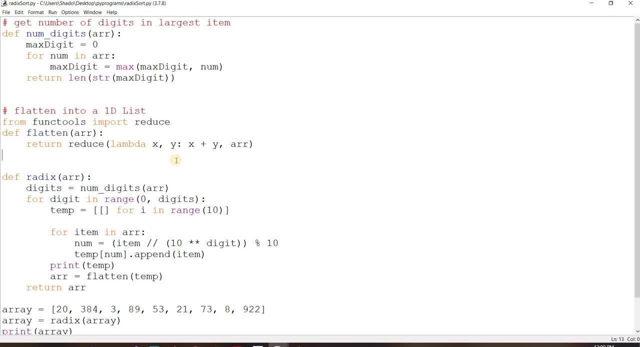 digits. So that also helps, because the smaller the number is, the less number of passes you'll actually require. OK, So, yeah, OK, So this has gone on long enough. There's some extra information on radix sort. There's some extra information on radix sort available in the actual website. 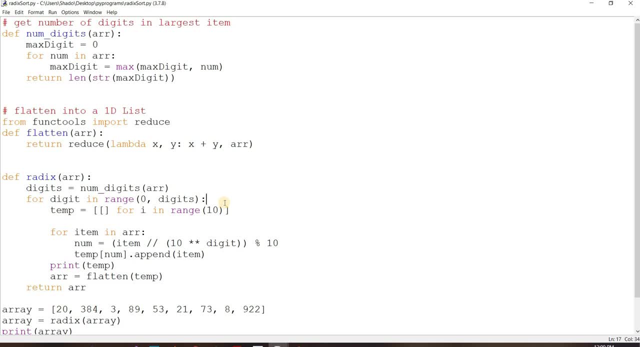 I'm actually adapting this from my actual website. All right, This is a video version of the tutorial over there, So there's some extra information available there, like best case scenarios, the big old notation time, complexity and a few other things.